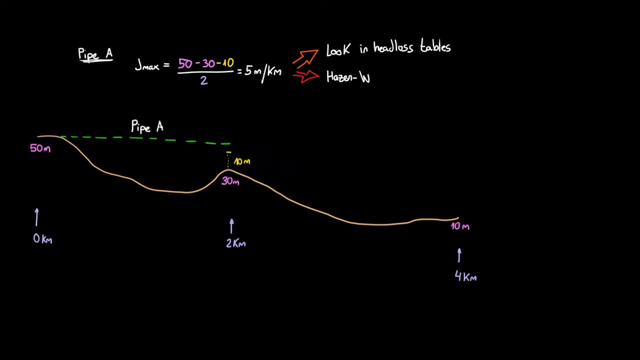 You could look in the pipe manufacturer's head loss tables, or you could look in the pipe manufacturer's head loss tables, Or use the Haysens-Williams equation. Since you need to know the internal diameter of pipes to use this equation, I find it's just more practical to read the values from the tables. 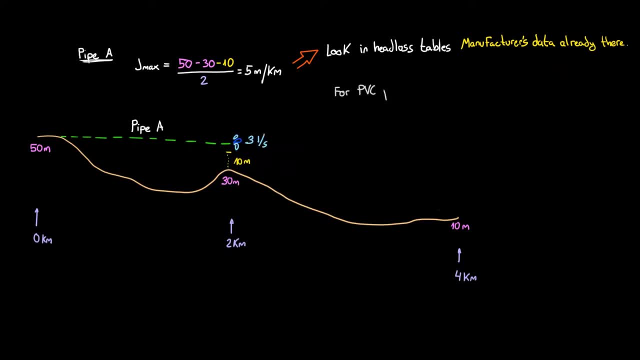 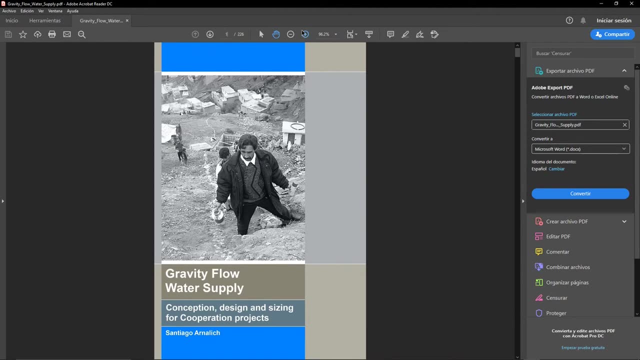 So let's have a look at the tables to see what pipes we could use for 3 liters per second. There are head loss tables in my books and there's also a download link in the video's description. There's a different table for each material. The 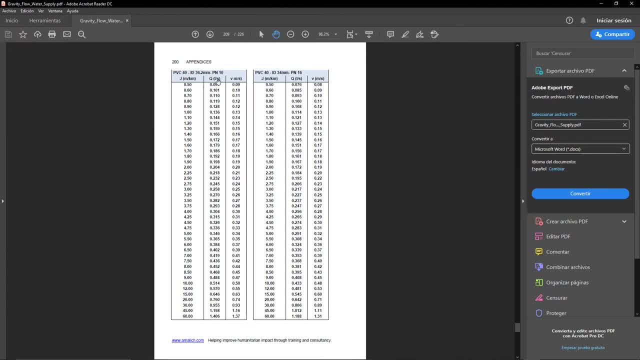 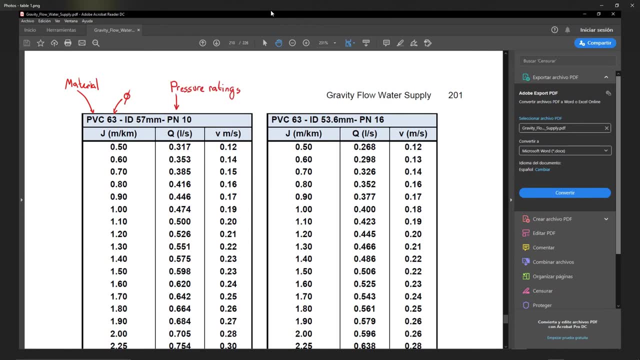 first one is the pressure rating. In this case I choose PVC, and since the maximum pressure is 40 meters or 4 bar, I will install 10 bar pipe PN10.. Then the head loss values are listed for increasing flow values. 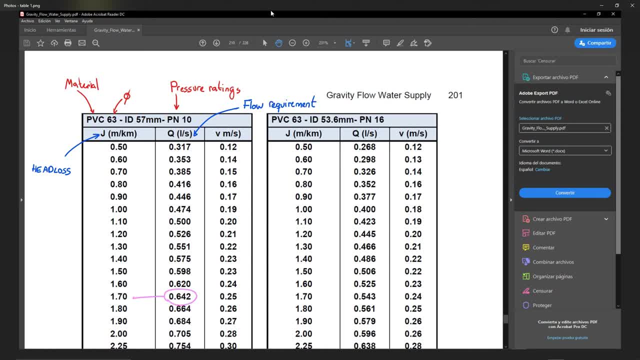 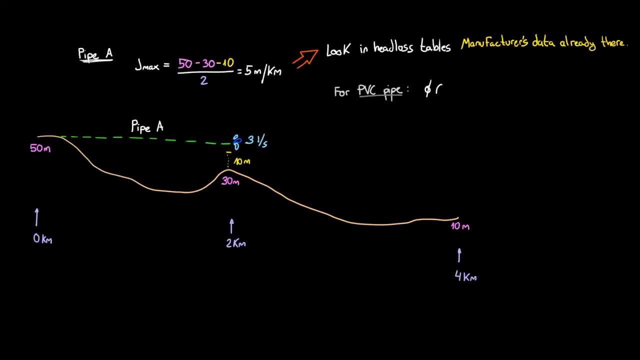 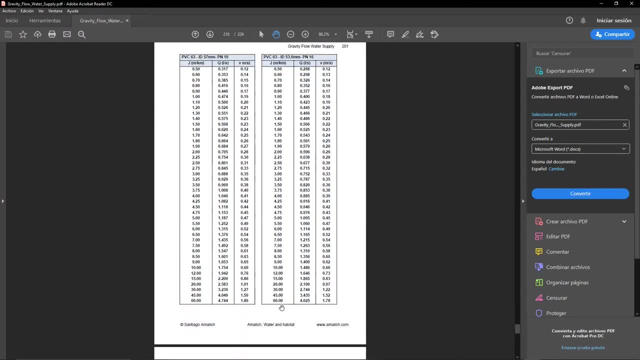 For example, 0.64 will cause 1.7 meters per kilometer of head loss. I will start tentatively with 63 millimeter pipe, the absolute minimum diameter I should install in a system other than house connections. My flow requirement, 3 liters per second, falls between values. 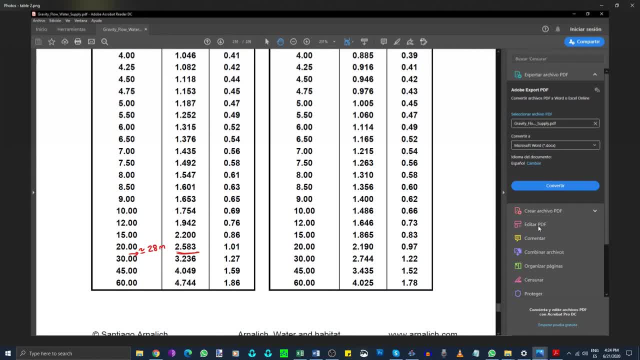 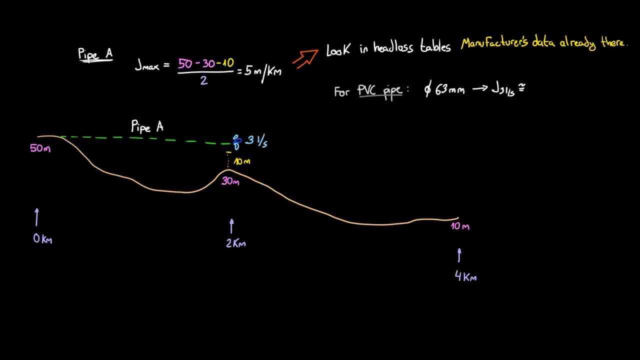 so I take it to be more or less 28 meters. There's a precise way to find this value, but let's leave that out for now. 28 meters is way more than the 5 meters per kilometer maximum value we calculated, and it will bring the line crushing to the ground. 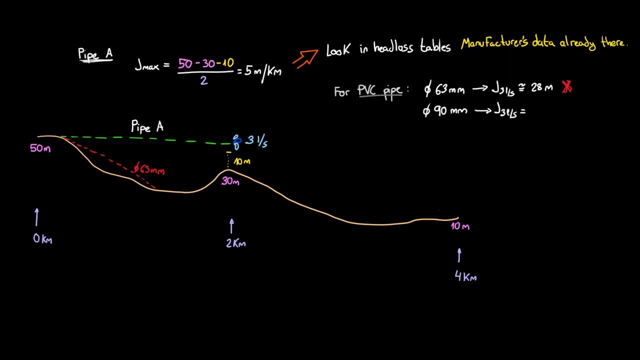 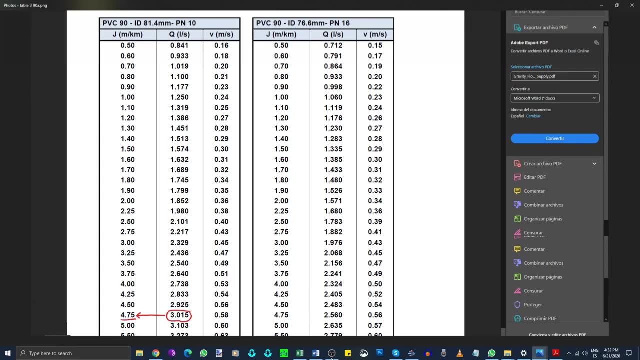 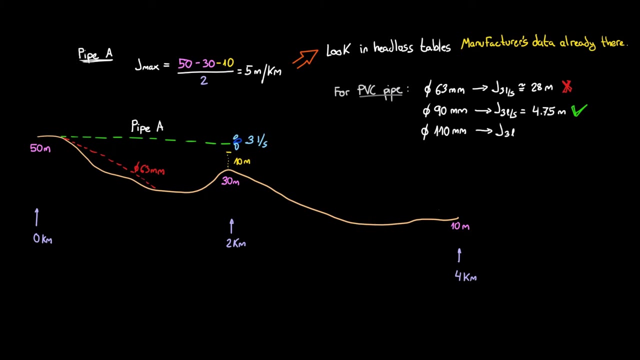 The next diameter is 90 millimeters. We read 4.75 millimeters. It is less than 5 meters per kilometer for 3 liters per second. It is less than 5 meters per kilometer and works. We read yet again another value for 110 millimeter pipe. 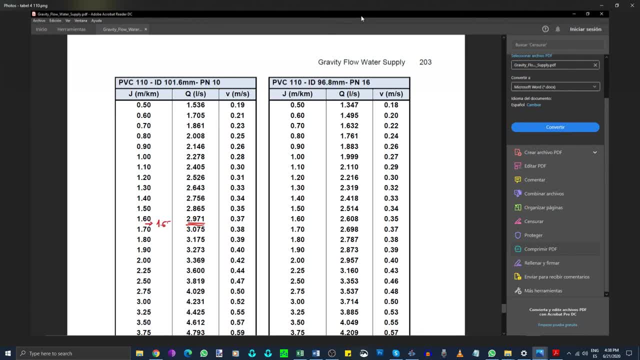 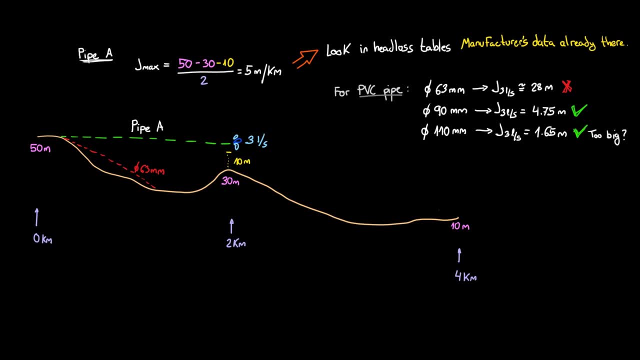 Again, it falls between values and we take it as 1.65.. The pipe will work, but it is more expensive. The best alternative seems to be 90 millimeters. Now the question is: what is the pressure at this midpoint? The difference of elevation: 50 minus 30, minus the losses, 4.75 over 2 kilometers.